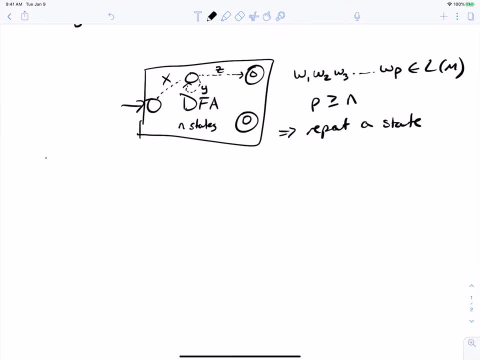 to the final state, We'll realize that if we look at the string x z, well, that just involves not going around that loop anymore. So this is also in the language. x y z is in the language also, because that's the original string. But if I do x y y z, that's also in the language. 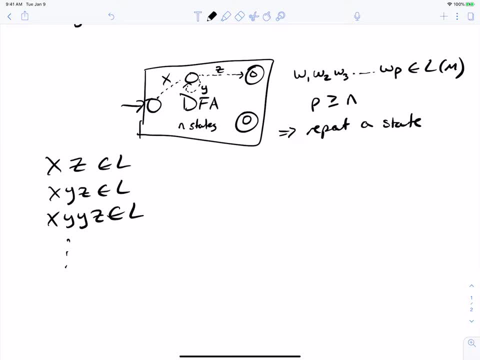 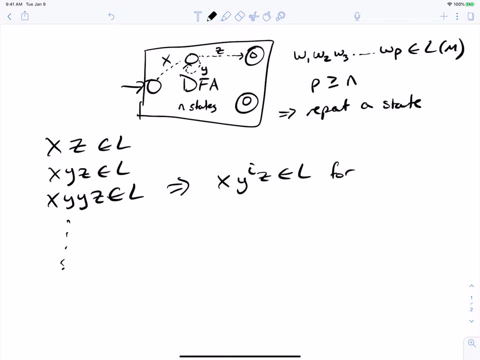 because that goes around the loop twice, And we can carry on like this to show that x, y to the i, z is in L, for all i, at least zero. Okay. Now, one thing we should also realize is that for the y bit, and only the y bit, 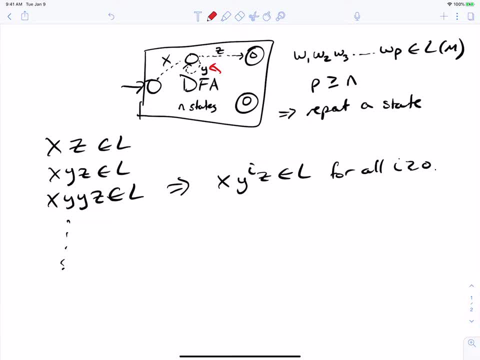 well, that involves at least one transition. because we have a DFA and we see the state twice, And because it's a DFA, each transition must involve a character. So we can immediately deduce from this that the length of y is at least one. 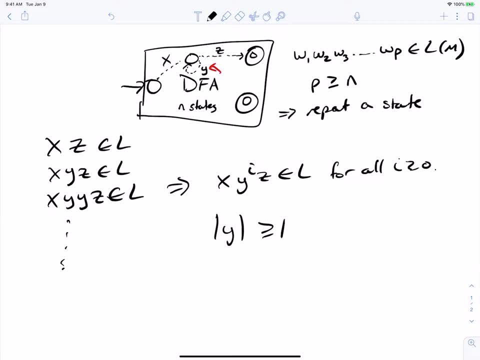 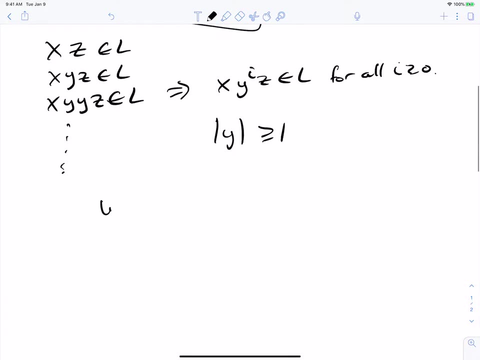 because it can't be zero, since we have a DFA. And if it were zero then that would involve an epsilon transition, but a DFA doesn't have any of those. Okay, So then, what else can we assume? Well, if we look at that string, that we had w1 up to wp, and let's just say that we 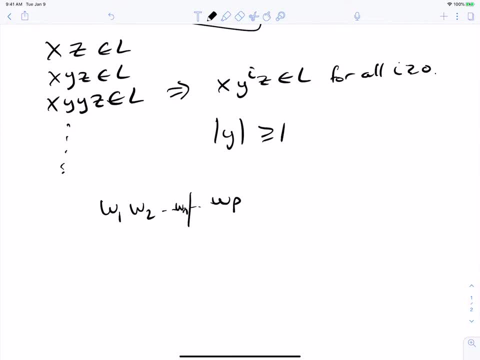 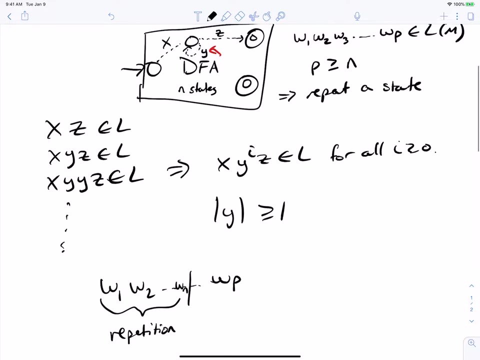 take the first n characters out of it. So remember, we have n states and let's just say we take the first n characters, maybe not, and not the entire string. Well, for the same reason, we can get a repetition in this part, because if I happen to have exactly n characters, then I would get a. 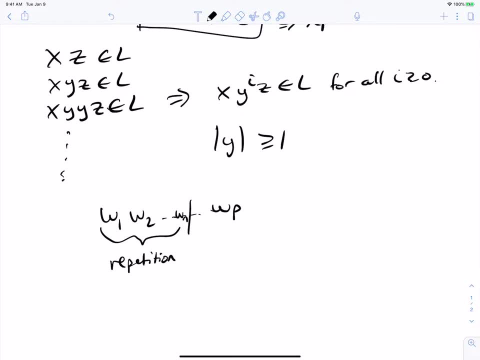 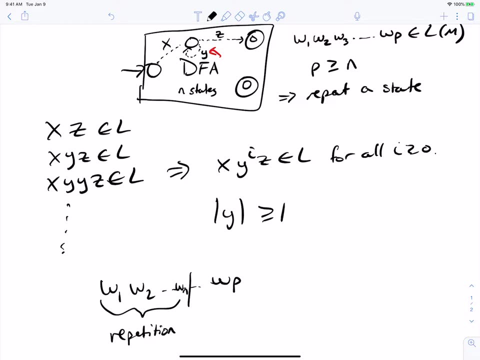 repetition anyway. So the repetition occurs within the first n characters. Well, what is the repetition part? It's the y string. So that means that x combined with y, where y is the first time a state in in the computation, repeats. Well, that means that the x and the y part are within the first.